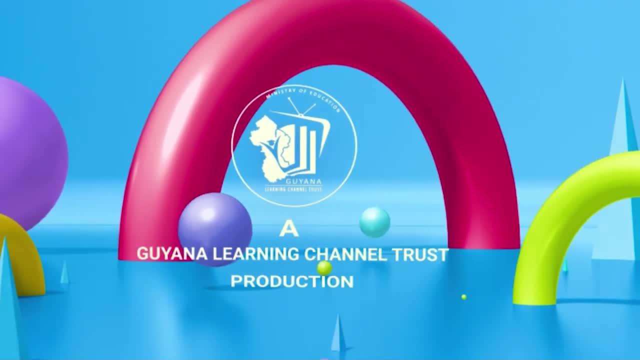 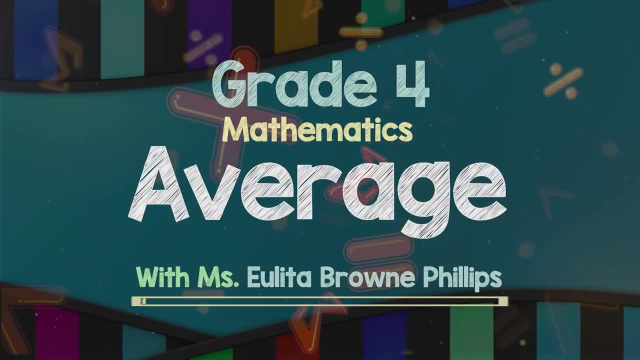 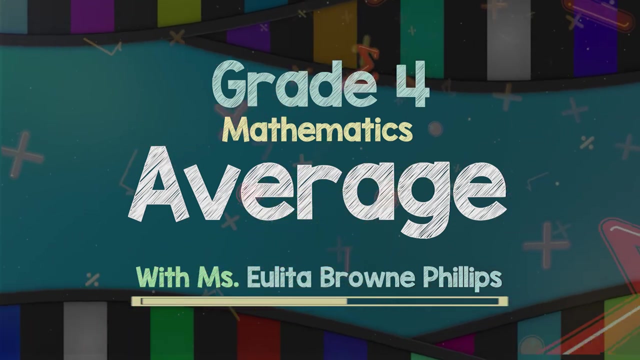 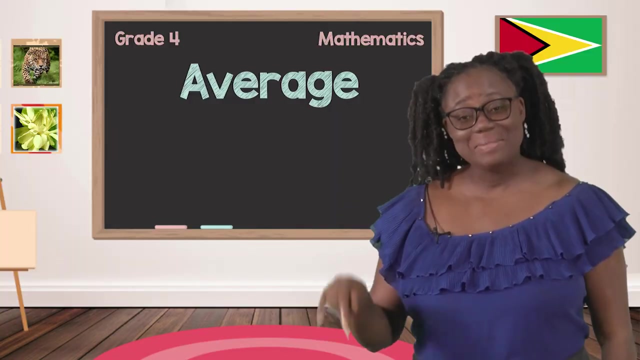 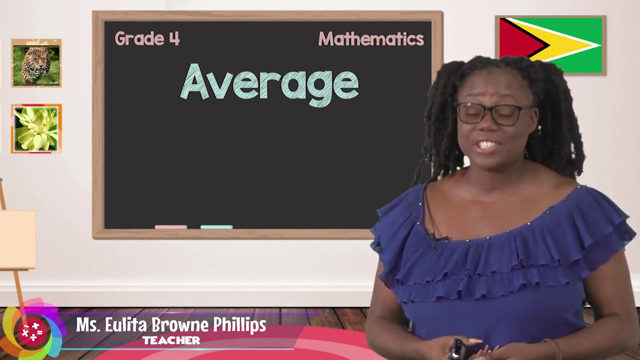 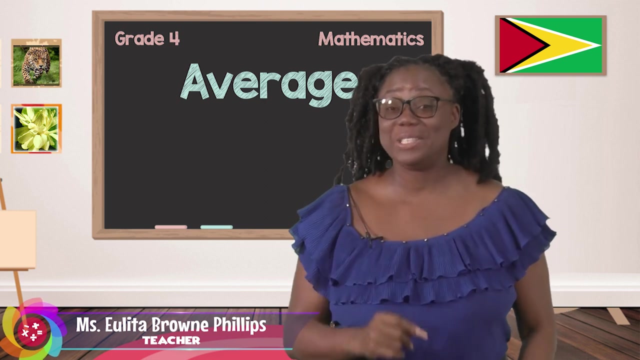 Hi, Team Grade 5!. Welcome to our mathematics class today And, as usual, taking you through the adventures in mathematics, I am your truly Missy Little Brown-Phillips. I hope that you are constantly tuning into the Guyana Learning Channel. 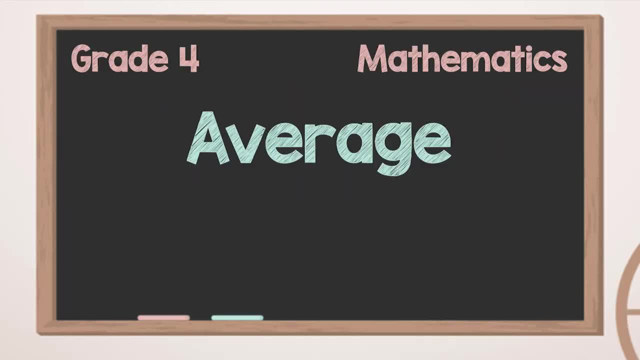 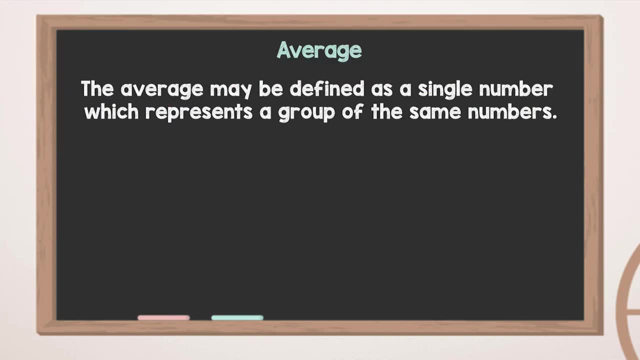 So, boys and girls, our topic for today is average. Have you ever heard that word before? Average, What is an average? The average may be defined as a single number which represents a group of the same numbers. Average is also known as mean. 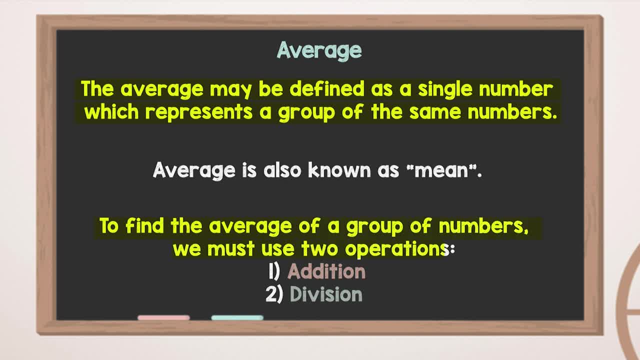 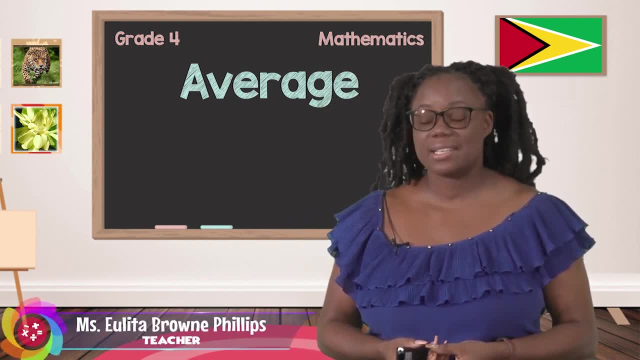 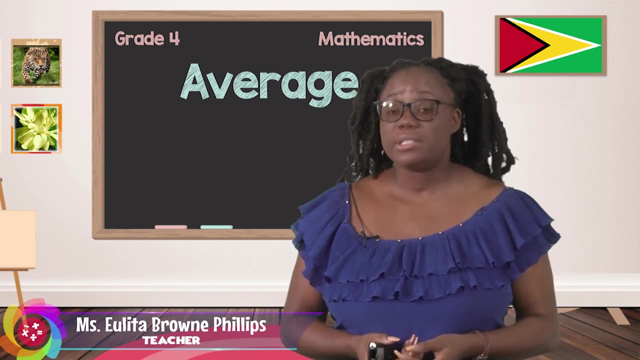 To find the average of a group of numbers, we must use two operations. We know that in mathematics there are four operations: Addition, subtraction, multiplication and division. However, to find the average, we will only utilize two of those operations. 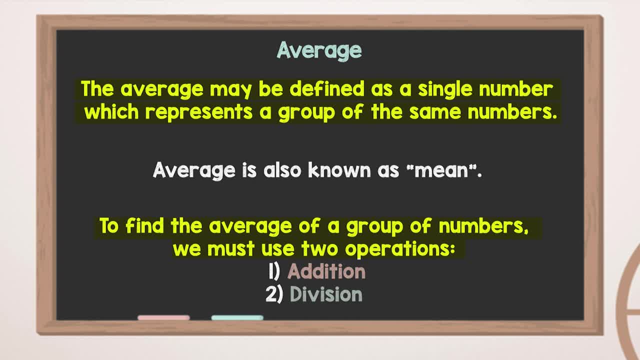 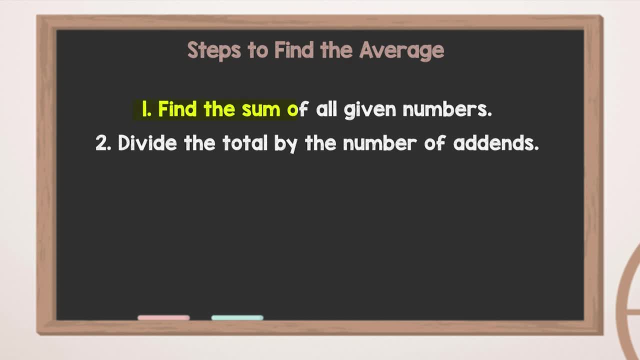 Addition and division. Let's examine the steps to find the average. Step 1. Find the sum of all given numbers. What is the keyword in that first step? that is, telling you what to do. Did you say sum? You are absolutely correct. 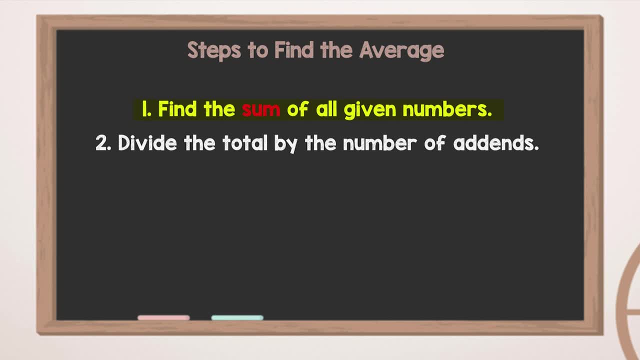 It means that you have to add Or find the total amount. Step 2. Divide the total- In this case it would be termed as the sum- By the number of addends. What are the addends? The addends are the numbers that you combine all together to get your total. 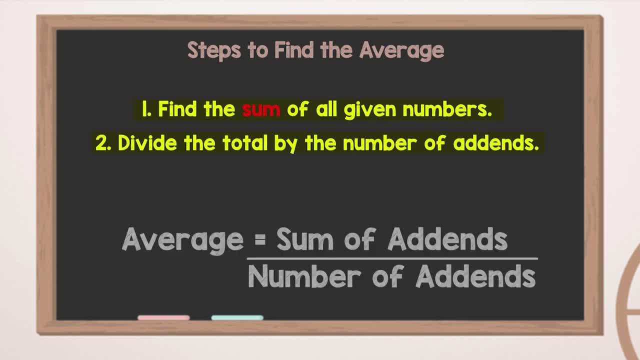 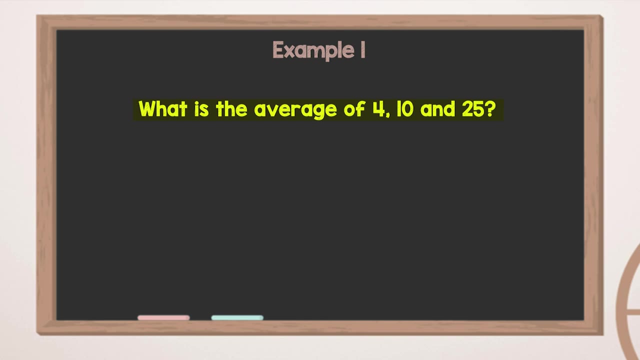 Let's write a formula to represent what we just said. Average equals Sum of addends Divided by number of addends. Easy, right. Let's run on quickly to an example. What is the average of 4,, 10, and 25?? 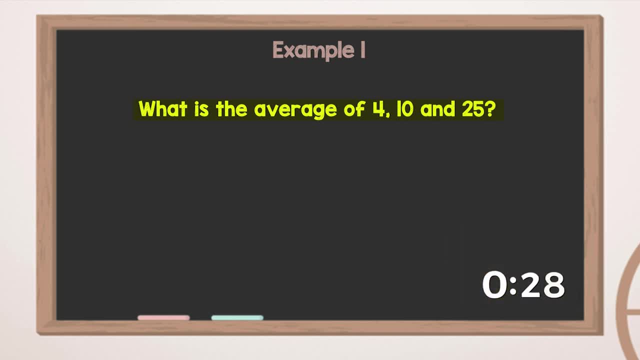 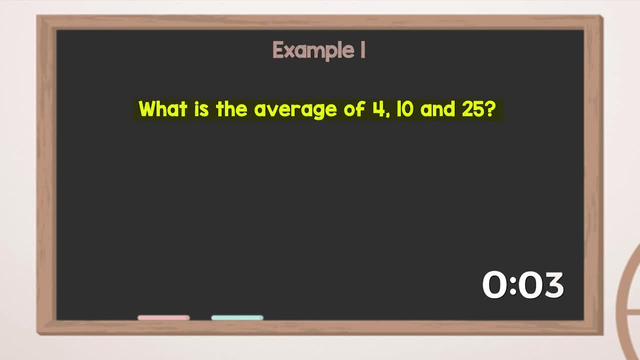 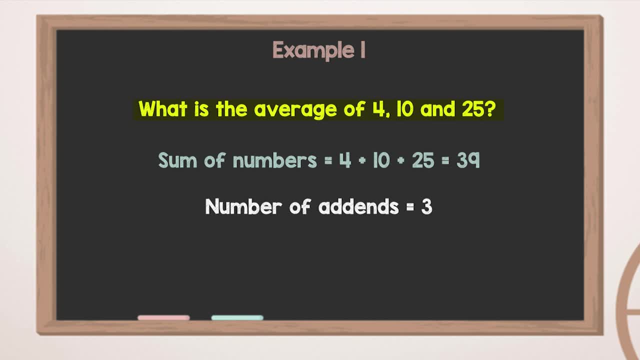 three numbers. so we have three addends. Average equals sum of addends 39, divided by number of addends 3.. 3 into 39, 13,, because 13 threes are 39.. Notice, you had to know your tables. 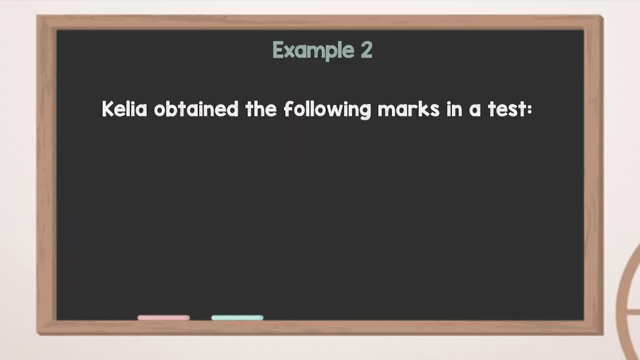 So let's move on to another example, This time a worded problem. Kelly obtained the following marks in a test: Maths 94.. Science 88.. Social studies: 86.. Language: 84.. Calculate Kelly's average mark. 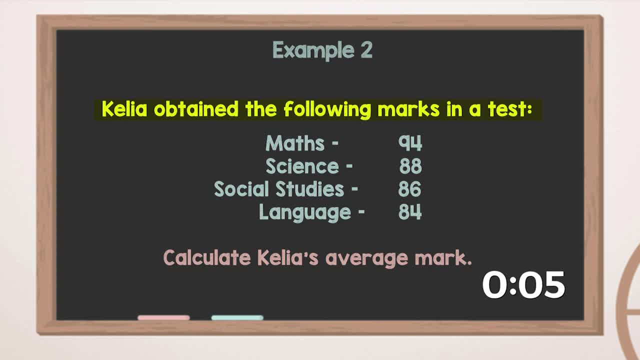 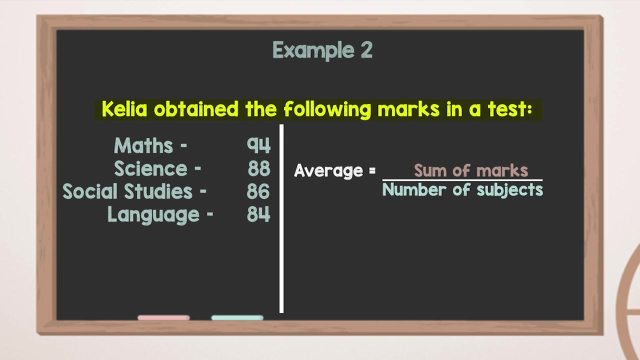 What did we say is? the first step to finding average? Find the sum of all given numbers. Step two: divide the total by the number of addends. So average equals. remember to always rewrite your formula. It will guide you in your working. 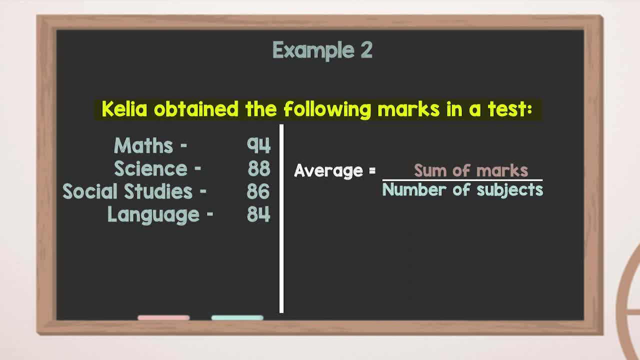 Average equals sum of marks divided by number of subjects. Sum of marks equals 98 plus 88 plus 86 plus 84. That will give us a total of 352.. Number of subjects: 4.. So average equals sum of number. 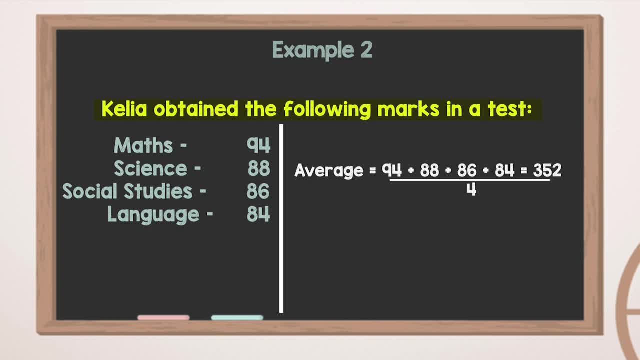 352.. Number of subjects: 4.. So we have to divide 352 by 4.. So this is a big number. Let's work a short division. How many times can 4 go into 35?? 8, because 4, 8's 32 and 3. 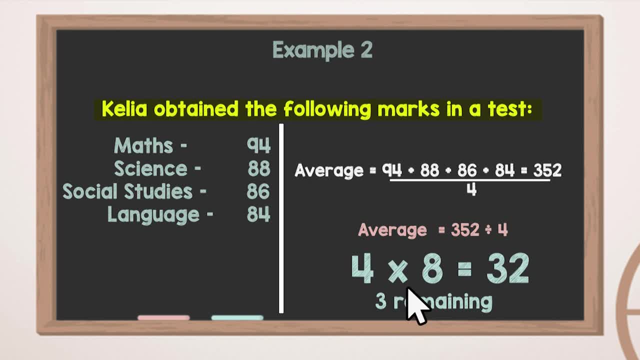 remains. So we put the 3 near to the 2 that is left there. So we have 32 divided by 4.. 4 into 32, 8.. So the average is 88 marks. Therefore Kelly's average mark in the test. 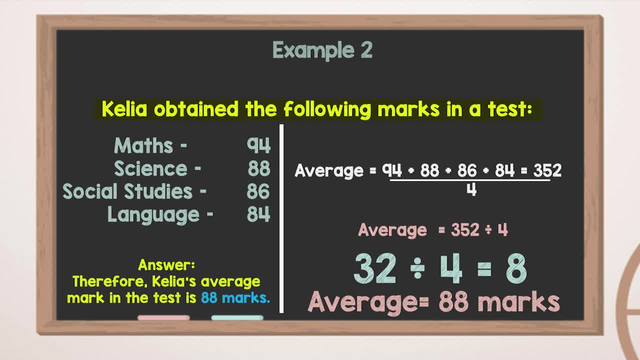 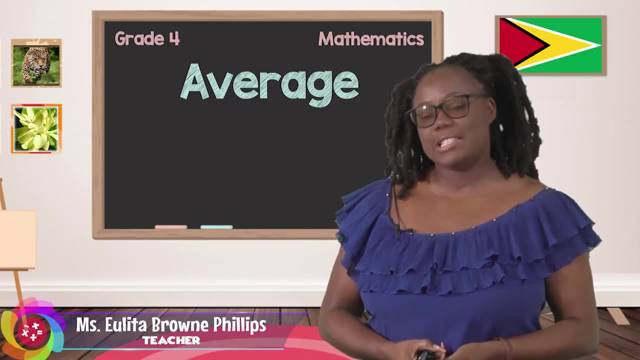 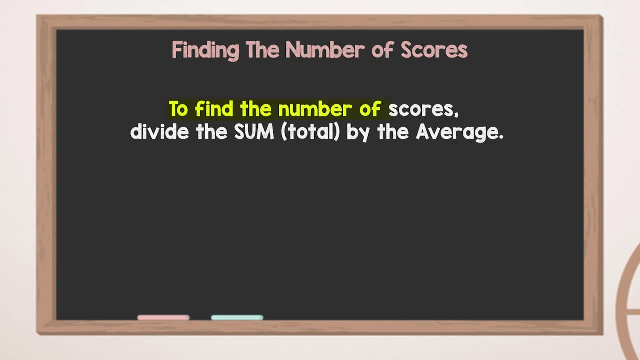 is 88 marks. Boys and girls. pretty simple, Don't you think? So? let's examine another aspect of average, where you have to find the number of scores. To find the number of scores, you divide the sum or the total by the average, So you will. 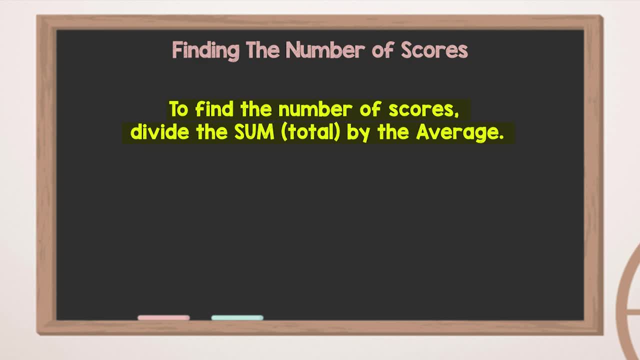 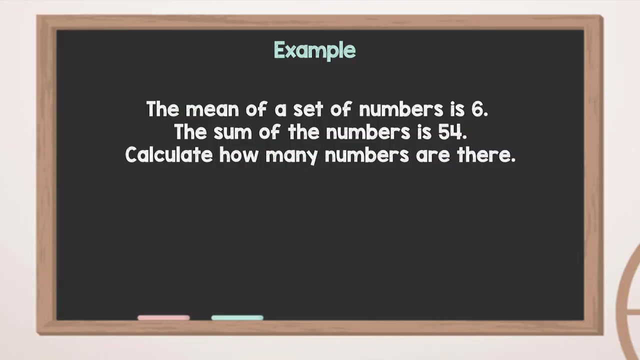 be given the sum or the total of the numbers and you will also be given the average To find out the number of scores. So let's write a formula for that. Amount of numbers equals sum divided by mean. Again, amount of numbers equals sum divided by mean. Let's look at this example: The mean of a. 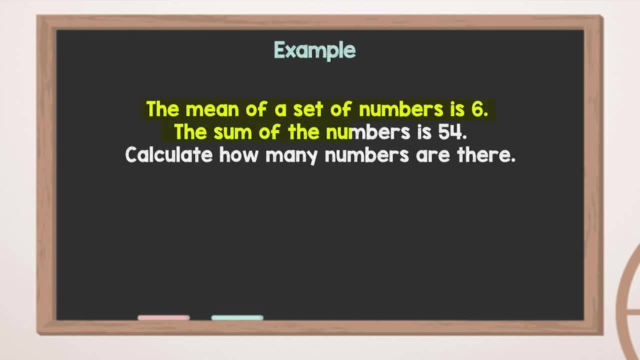 set of numbers is 6.. The sum of the numbers is 54. Calculate how many numbers are there. Thank you. Now, boys and girls, remember we said that when we want to calculate the amount of numbers or the amount of scores, it is the sum divided by the mean. 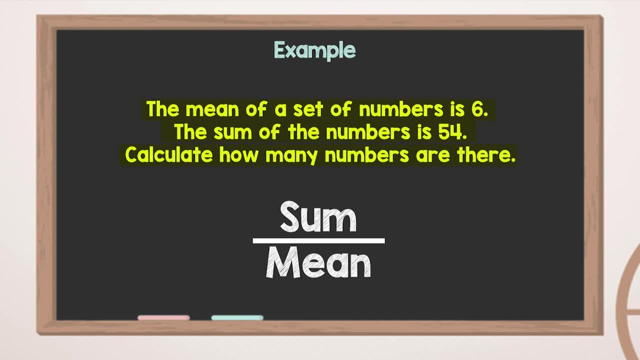 So in this case, amount of numbers equals sum divided by mean. What is the sum? 54.. What is the mean 6.. How many groups of 6 can you get from 54?? Or how many times 6 can go into 54?? 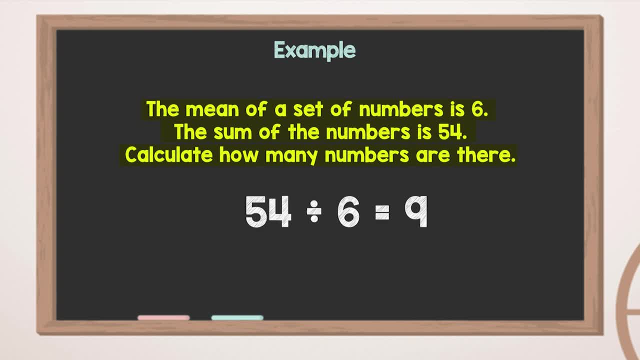 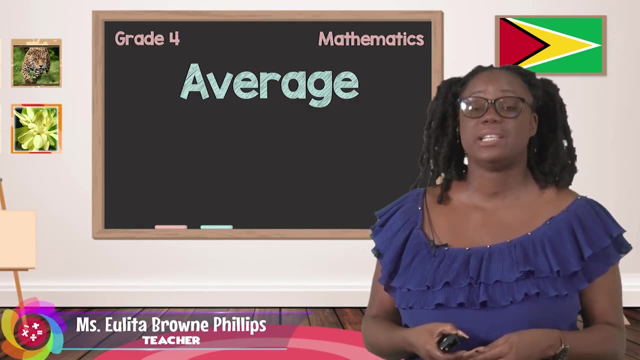 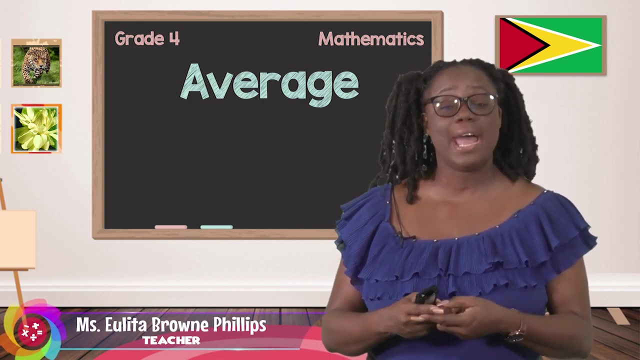 9, because 6 nines 54. Therefore, the amount of numbers that are there is 9.. Boys and girls. I hope that you would have understood this concept clearly. However, I still want to find out if you understood it by giving you an acronym. 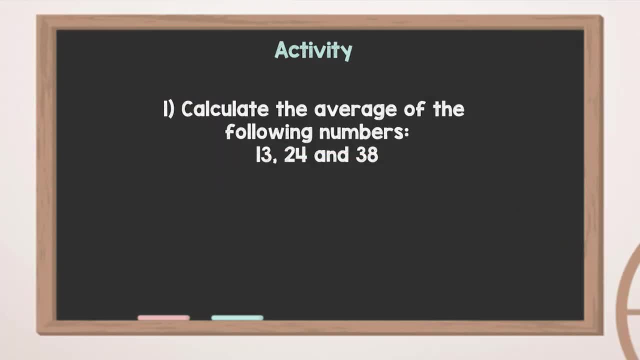 Let's quickly work this. Calculate the average of the following numbers: 13,, 24, and 38.. Boys and girls, remember the formula to find the average is: Take a minute and get this done. Remember to do neat work. Your work says a lot. 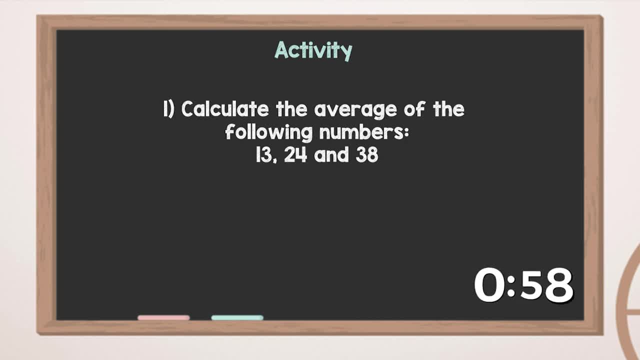 Arts about you, Doion Umı. What are you looking forward to, Dad? What ever you do, do not give up on the future or last year. Do not forget to click the caret responsibilities in the description below the video. I'll see you in the next video. 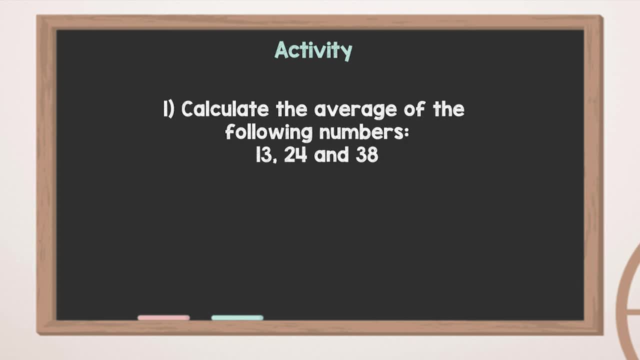 I'll see you in the next video. I'll see you in the next video. I am so proud of you. Number two: The mean set of numbers is four, The numbers added up to 36.. How many numbers are there, Boys and girls? remember when you have to calculate the amount of numbers or the amount of scores. 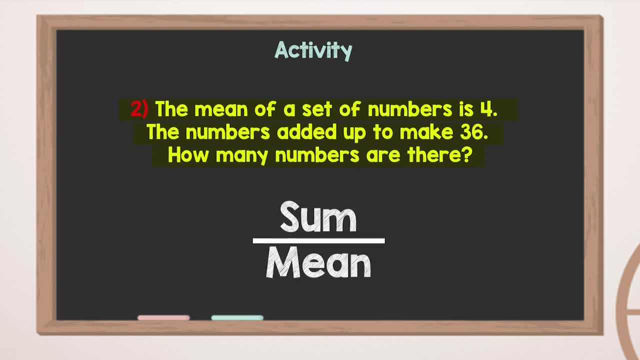 you use the formula sum divided by mean. Take a minute and get this done. Come and do it, although you're not quite ready. I'll see you in the next video. Buh, oh, I'll see you in the next video. 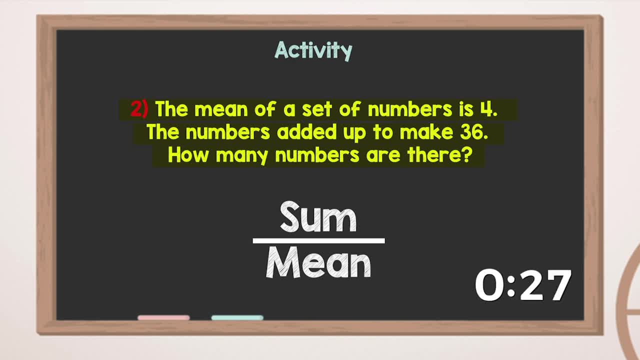 Bye, Bye, Thank you. You should be finished by now. I'm so excited to see how you work this problem. So amount of numbers equals sum divided by mean. What is the sum of the numbers? Yes, 36.. What is the mean? 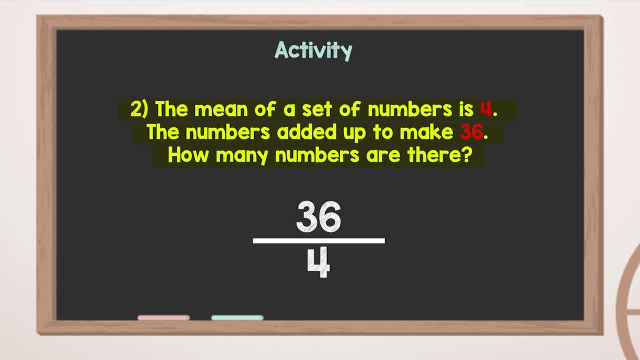 4. Boys and girls, did you notice that I used the word mean instead of average? In actuality, mean and average means the same thing. So never get scared if you open an exam paper and instead of seeing average, you see mean. 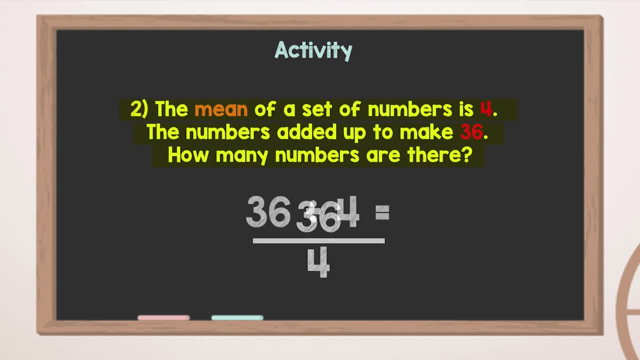 You know that it is the same thing. So 36 divided by 4. How many times can 4 go into 36?? 9. Because 4 nines equals 36.. Therefore, the amount of numbers that are there is 9.. 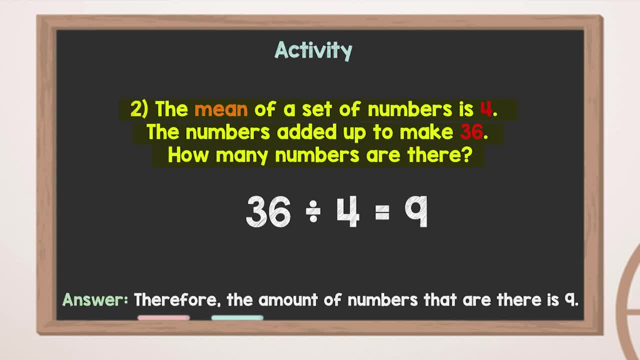 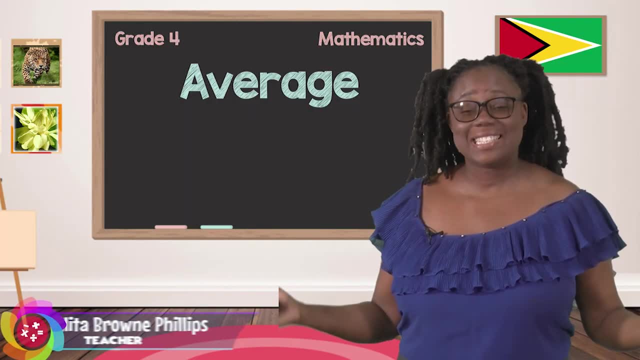 Boys and girls, do you have this problem correct? I want you to put a big tick. I am extremely proud of the work that you are doing. Boys and girls, let's take a break. It's trivia time. So for today's trivia, 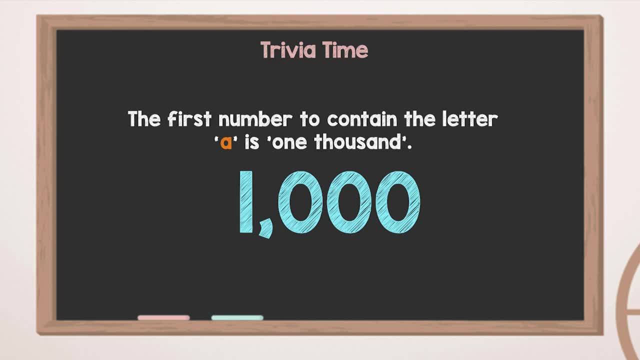 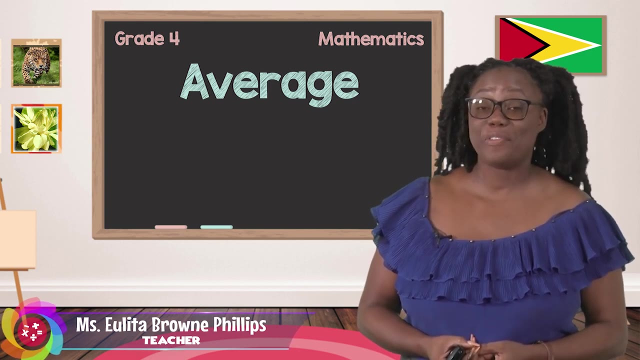 did you know that the first number to contain the letter A is 1000?? Yes, go check it for yourselves. So, boys and girls, you've learned quite a lot today, including that the first number to contain the letter A is 1000. 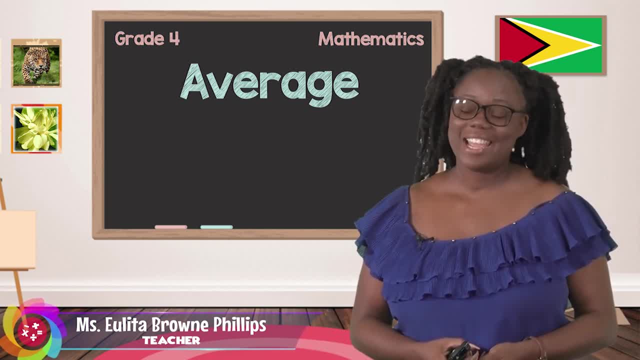 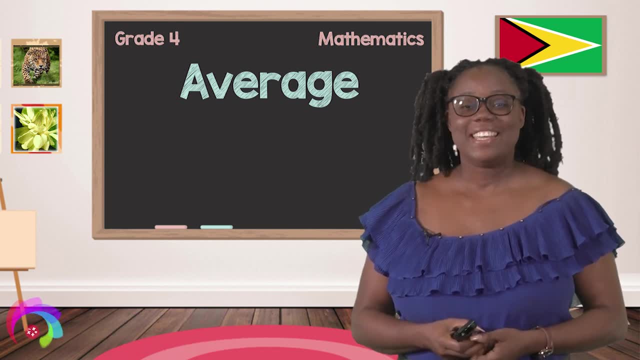 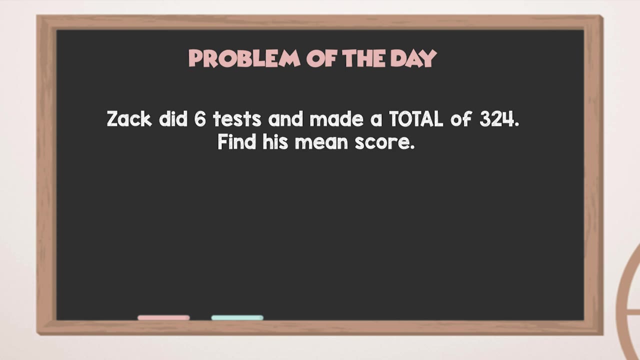 This has brought us to the end of today's class. However, we never end our class without knowing the answer, The problem of the day. So for today's problem, Zach did six tests. He made a total of 324.. Find his mean score. 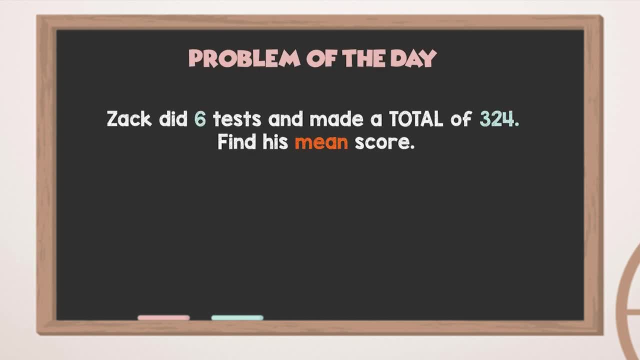 Notice the word. mean: Take a minute to get this done. boys and girls, I am so excited. Remember to do neat work. Your work says a lot about you. I am so excited. Your work says a lot about you. So for our solution. mean: equals sum of scores divided by number of scores. 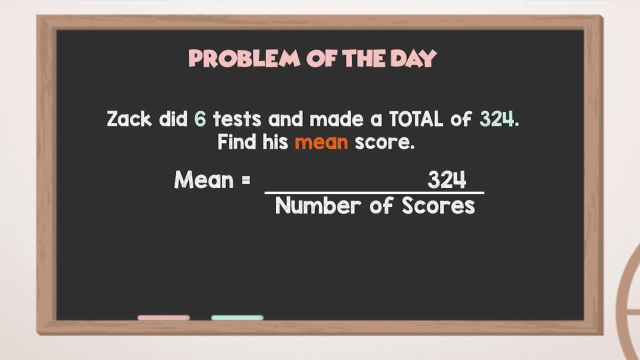 Mean equals 324.. That is the sum of the scores. Remember it was given the total of 324.. Number of scores: six, Because Zach took six tests. So let's divide Three hundred twenty-four by six. We're going to do short division. 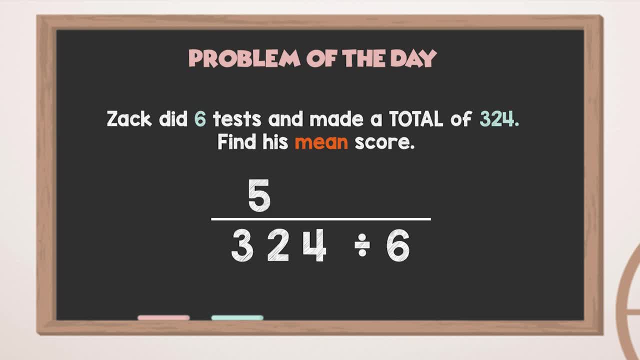 Six into thirty-two five, Because six, fives thirty And two remains. So that leaves us with twenty-four. Six into twenty-four four. Therefore, Zach's mean score is fifty-four. Boys and girls, do you have that correct? 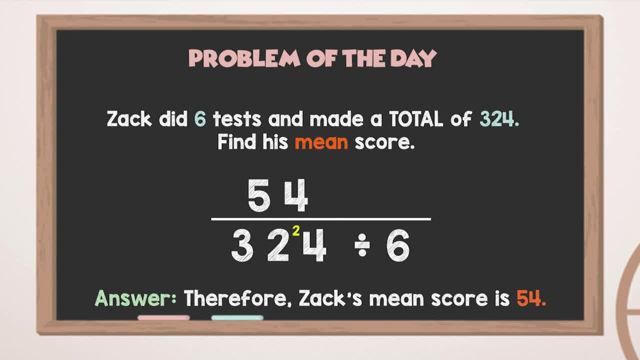 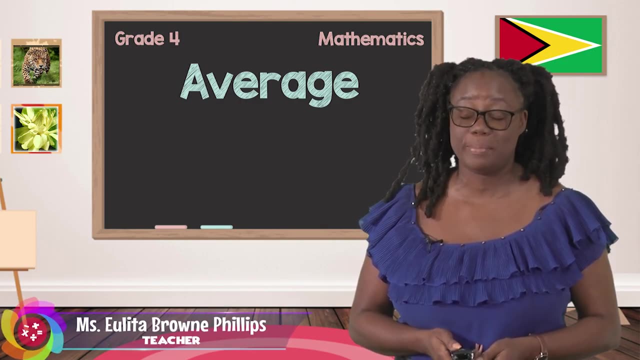 Excellent Put a big tick. I know that You'll never disappoint me and I can always depend on you to solve the problem of the day. Thank you, boys and girls, for solving the problem of the day for me. Thank you for joining me today.